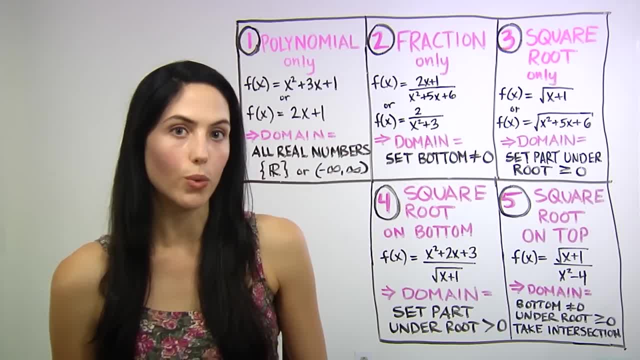 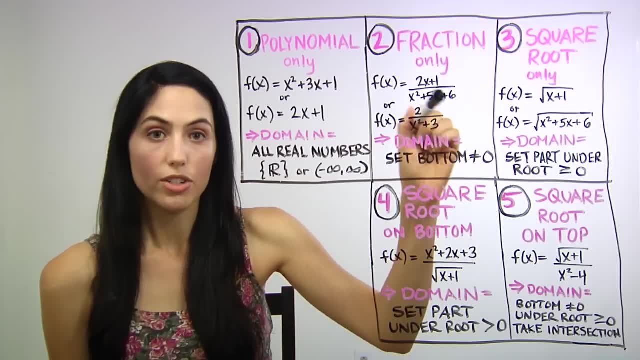 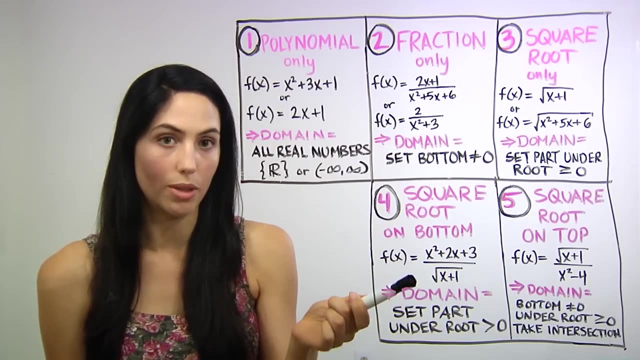 more complicated, like a fraction or a square root, or possibly both. it's going to be one of these four cases. It's either just a fraction. it's a square root on its own, it could be a fraction with a square root in the bottom, or a fraction with a square 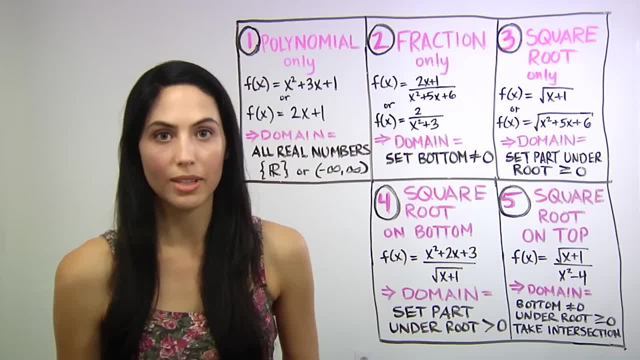 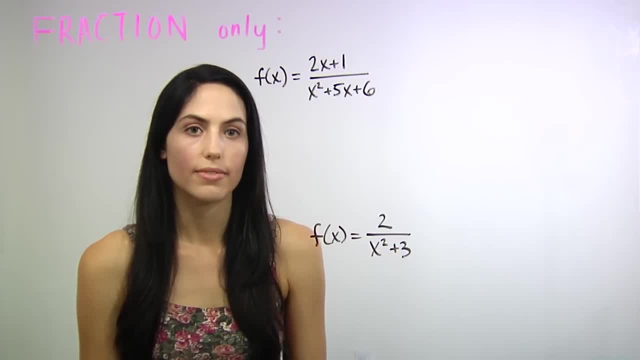 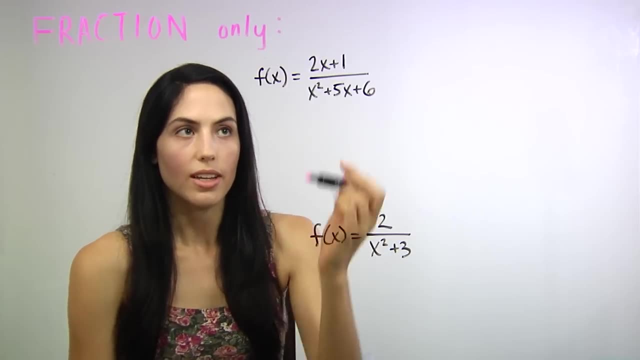 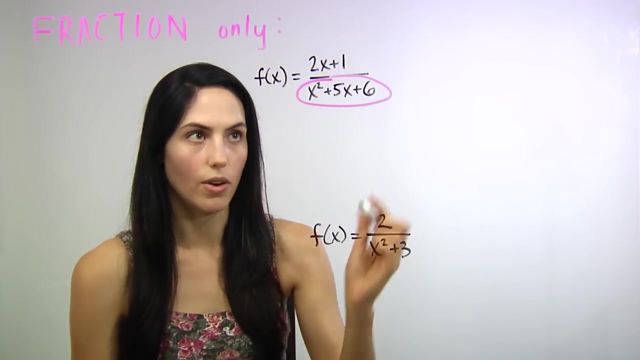 root in the top, the numerator, And I'm going to explain how to find the domain for all of those cases. Okay, Say, you have just a fraction. To find the domain, all you have to do is look up your set of numbers. What you want to do is take the bottom, whatever that may be, and 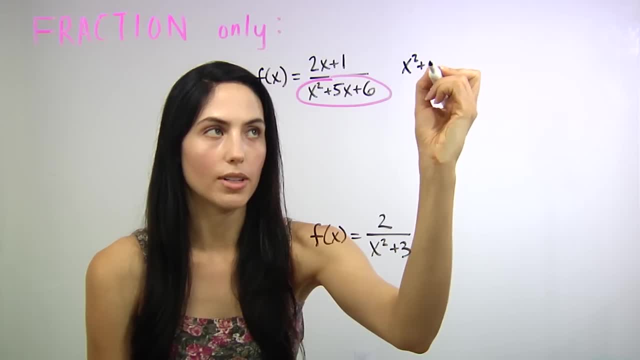 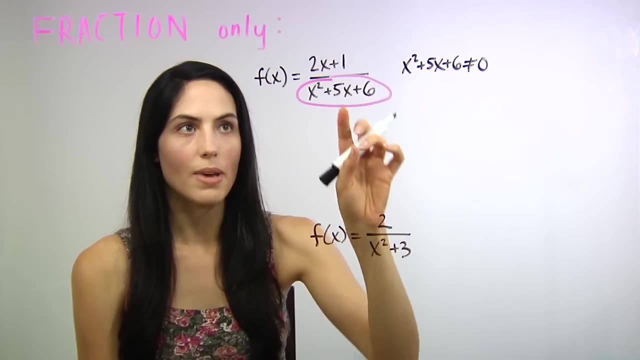 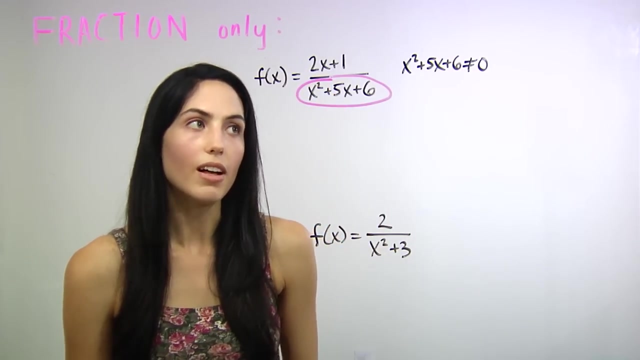 set it not equal to zero. So in this example we have x squared plus 5x plus 6, not equal to zero. Notice that it doesn't matter what the top is, just take the bottom and set it not equal to zero. And you can solve this just as if it were a normal equality, And that involves fine. All right, Let's talk about 6x and 6x Mobile lemmas. let's take this wing up. We're going to start with a lokmanopp sign: 1,, 2,, 3,, 4,, 4.. Okay, we're going to pick the bottom like this: 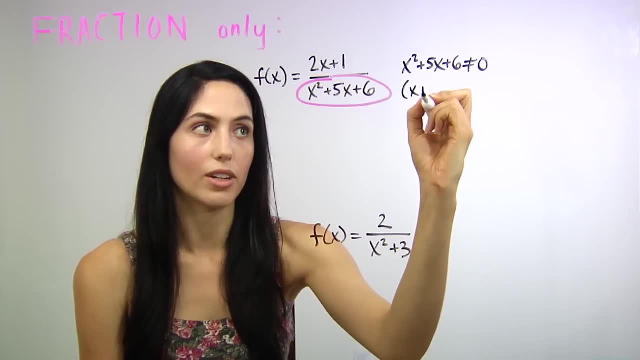 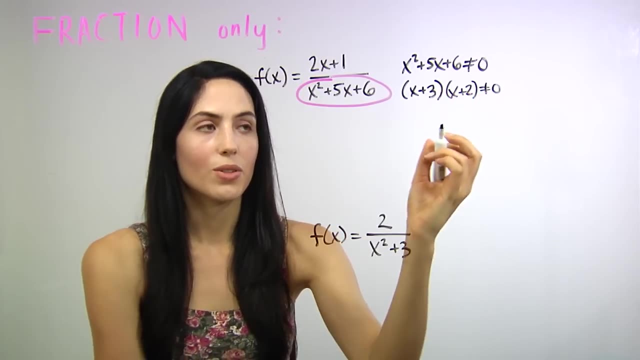 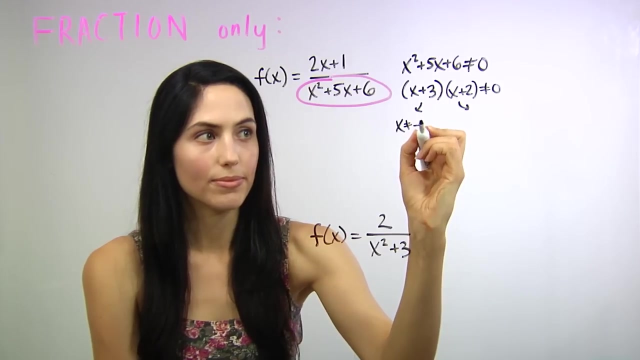 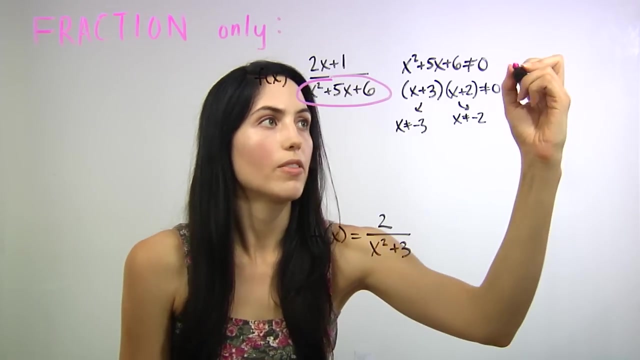 factoring. If you need help with factoring or solving by factoring, you can look at one of my other videos. So in this equation we get two restrictions, two solutions: x cannot equal negative 3, and x cannot equal negative 2.. So when we want to write the domain, the final answer: 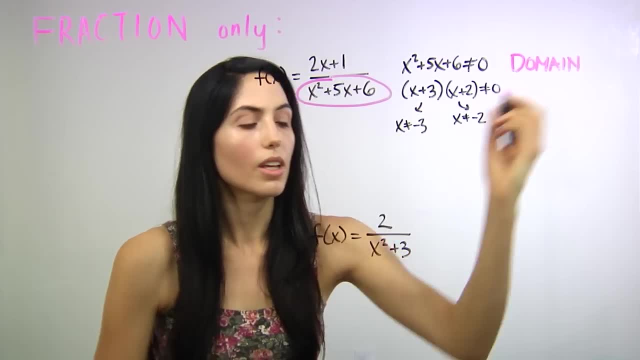 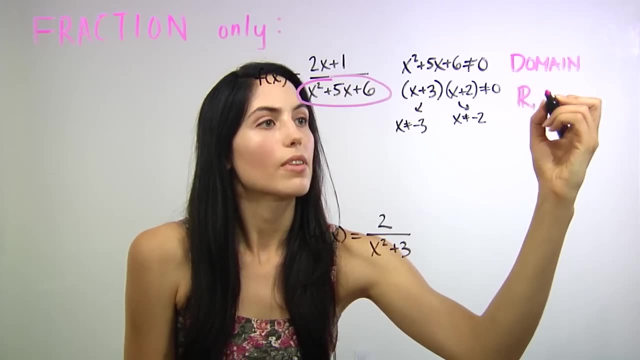 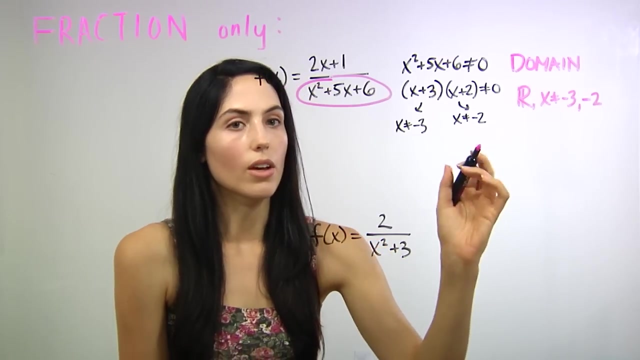 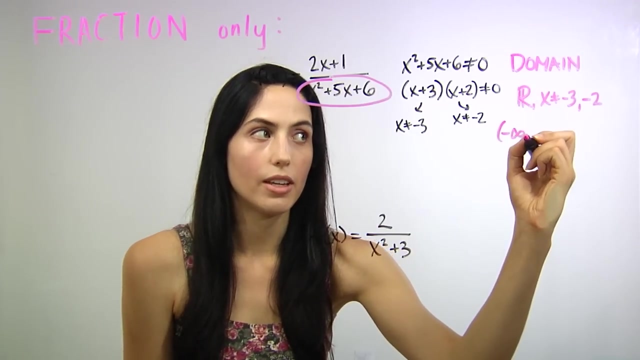 for domain. you can write it as all real numbers, but x cannot equal negative 3, and cannot equal negative 2.. Or you can use interval notation and write it as everything from negative infinity all the way up to negative 3,, not including negative 3.. 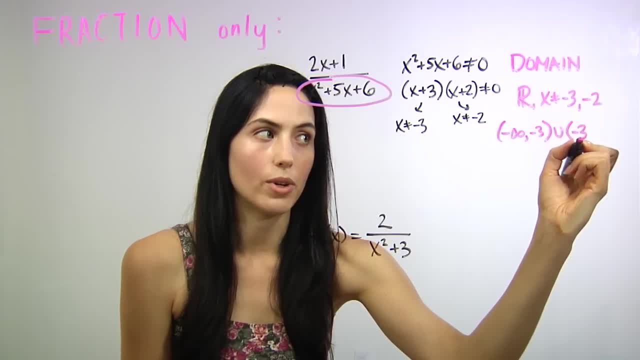 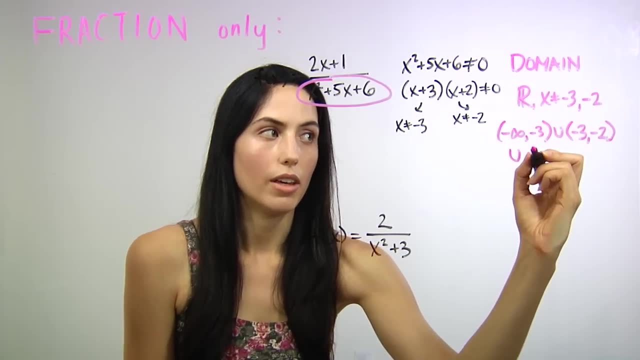 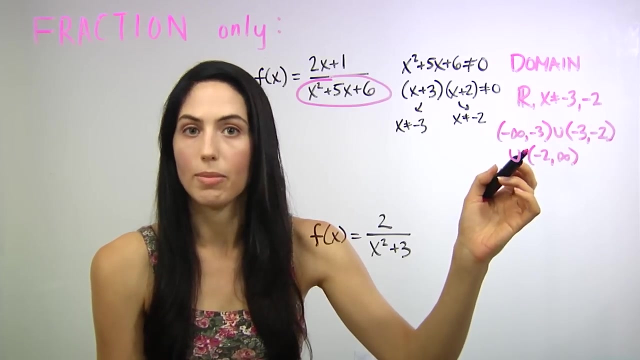 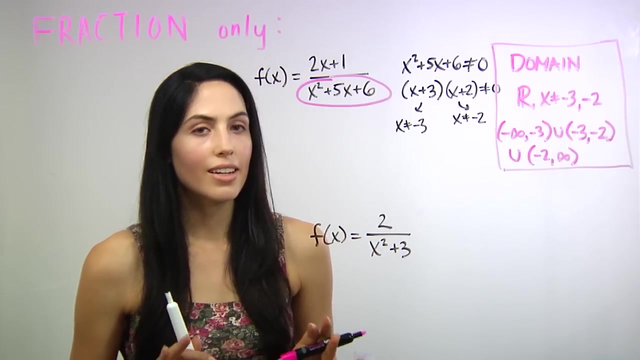 Combined with everything from negative 3 to negative 2, not inclusive of either number. Combined with everything from negative 2 all the way up to infinity. So either of these notations is fine. They mean the same thing. Let's look at another example. What if you're given something like this, where the denominator 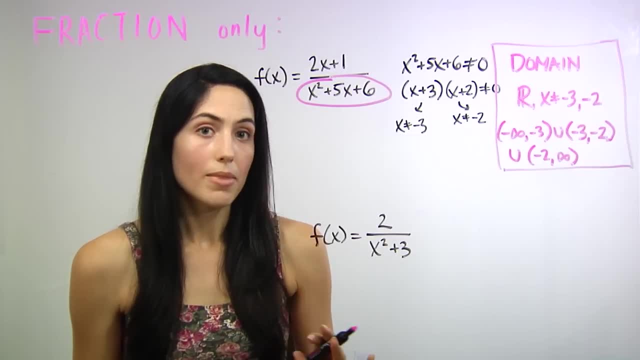 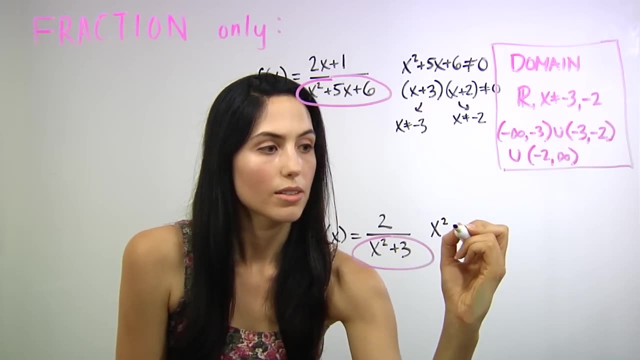 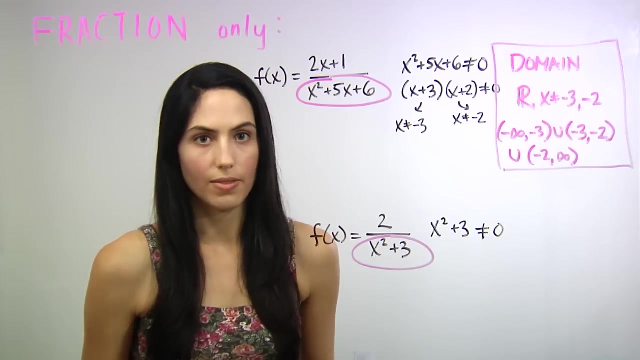 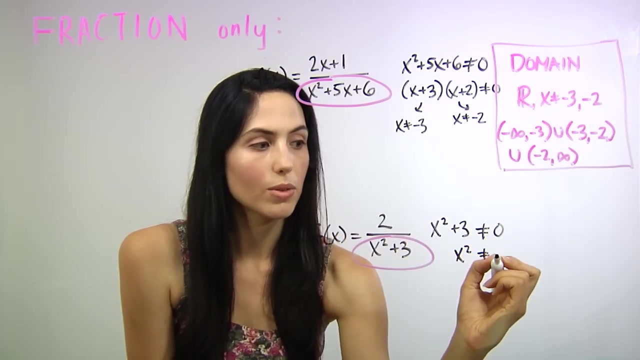 is x squared Plus 3.. Same thing. Take the bottom. Set it not equal to 0, because we cannot have the denominator equal to 0. It's not defined when it is. Now. when you solve this equation, you end up with: x squared cannot equal negative 3.. 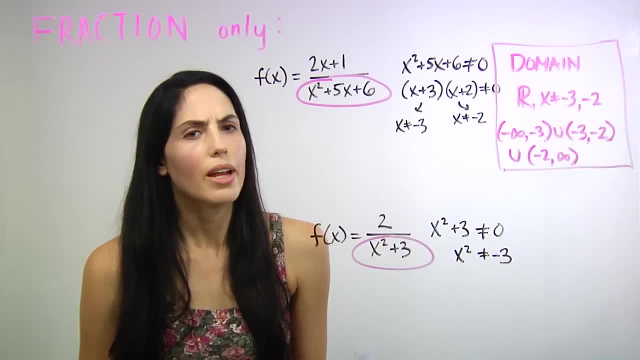 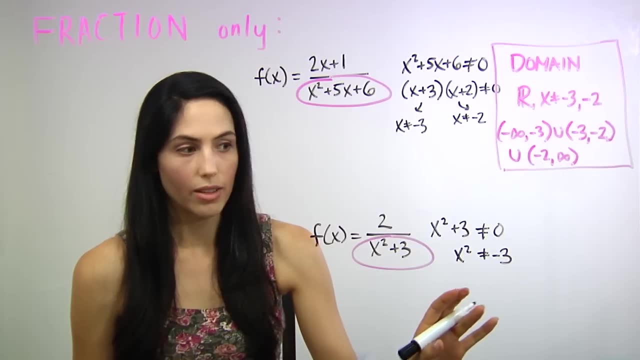 But x squared can't be equal to negative 3.. And if you're given the denominator, the denominator cannot equal negative 3.. It's not defined. when it is Now we can have, the denominator can never equal negative 3, so we just can't have that ever. There's no x value that would. 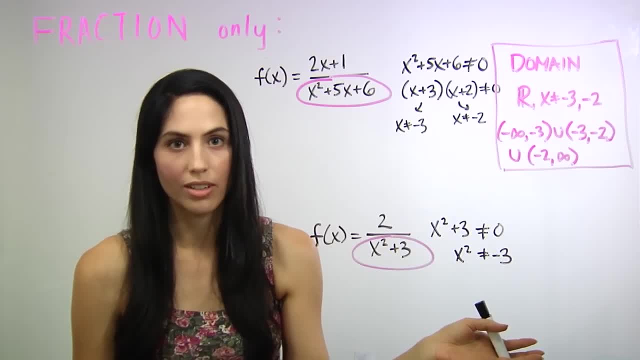 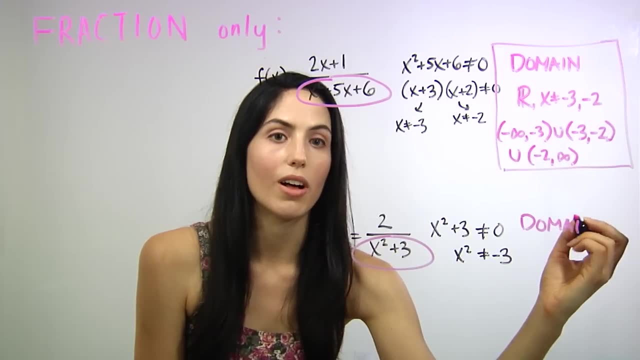 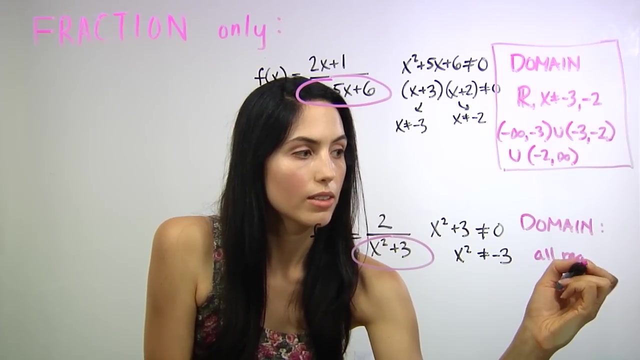 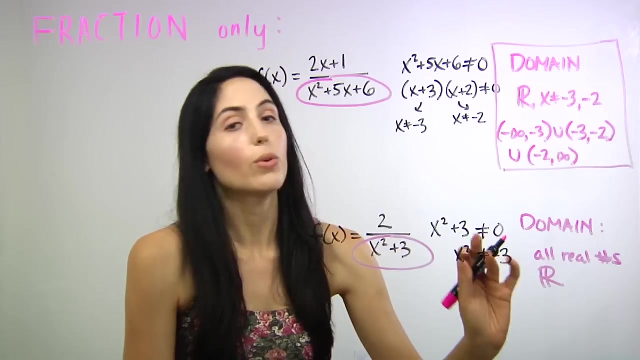 ever make that happen. so you don't need to worry about that restriction. All you need to write in that case would just be your normal all real numbers domain, So you can say all real numbers. you could say capital R symbol for all real numbers. or you could say with: 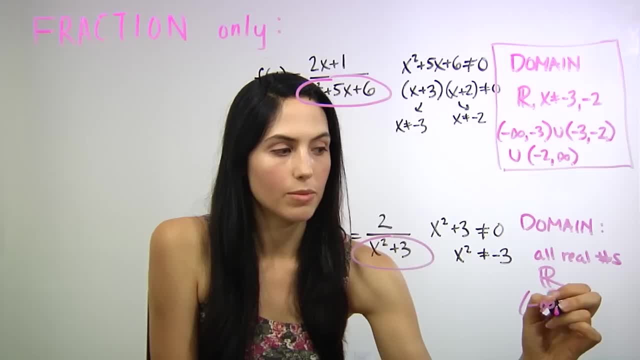 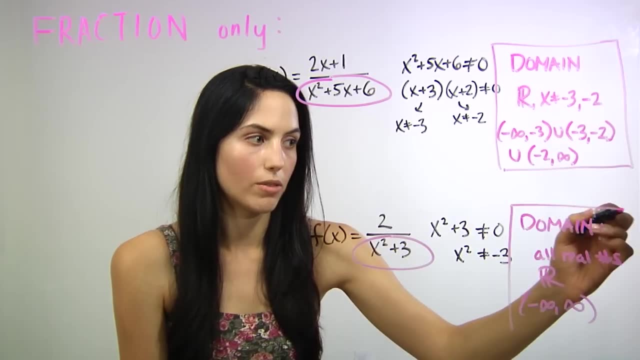 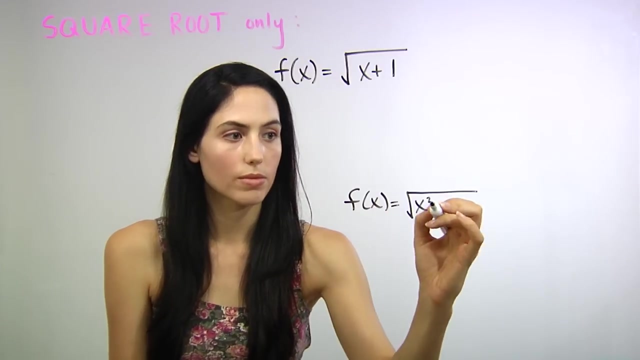 interval notation: everything from negative infinity to positive infinity, with parentheses on either side. So that would be your three ways of writing the domain for this fraction. Now let me show you what to do if you have just a little bit of time. If you have just a little bit of time, you don't need to write. 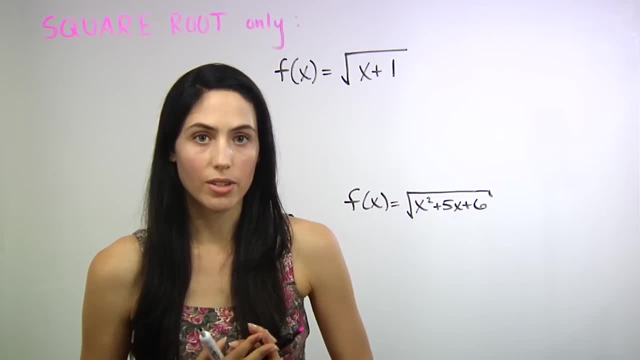 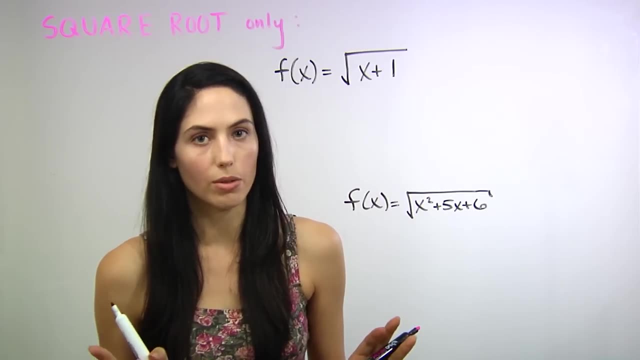 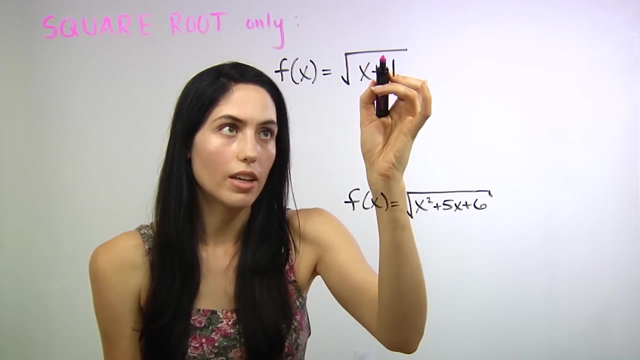 just a square root in your function. I'm going to focus on a square root, but this is true for any even root- fourth root, sixth root, etc. It's not true for odd roots like third root. If you have a square root or an even root, you take the expression underneath the 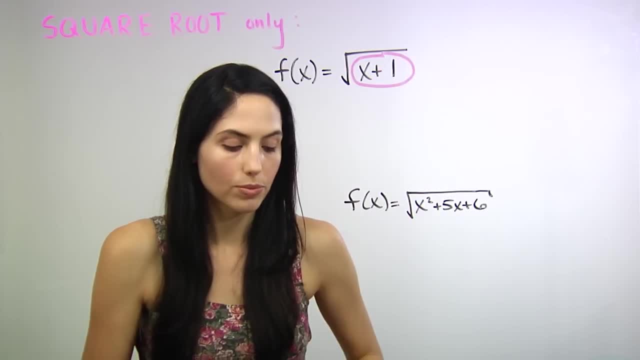 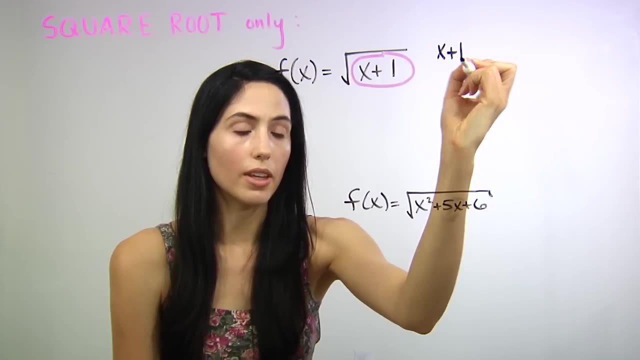 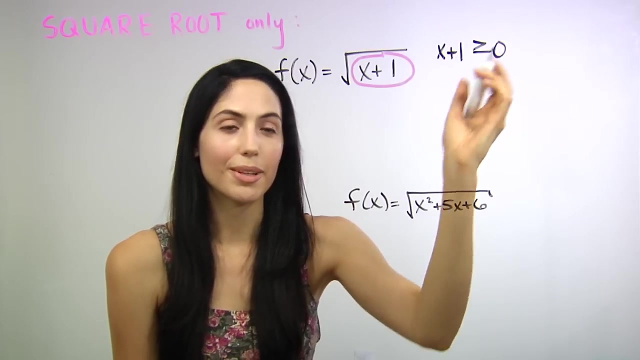 radical sign, which is the radicand, everything that's underneath the root symbol. so in this case, that's plus one, and you need it to be greater than or equal to 0. Because we can't have a negative number underneath a root. You can only have a positive number. 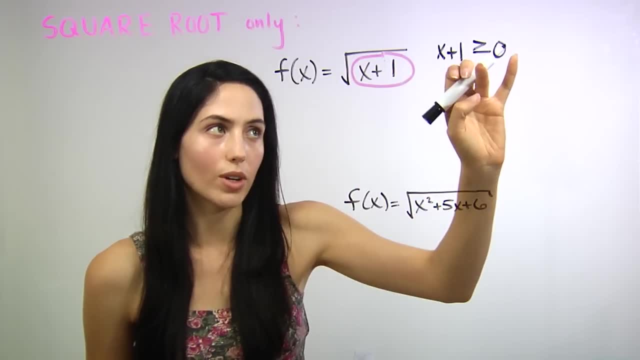 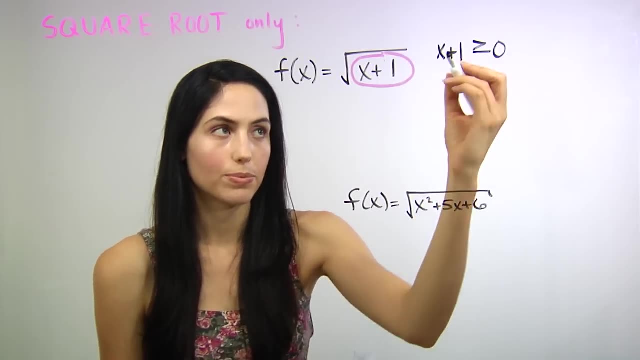 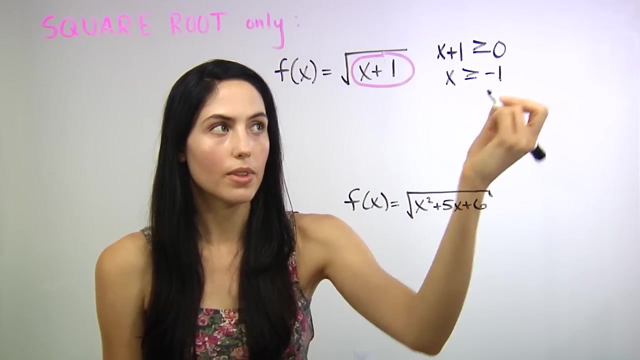 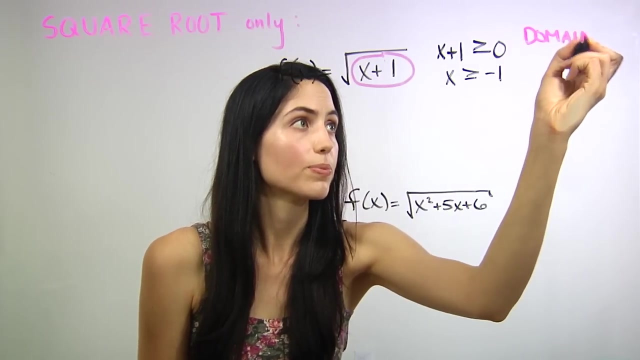 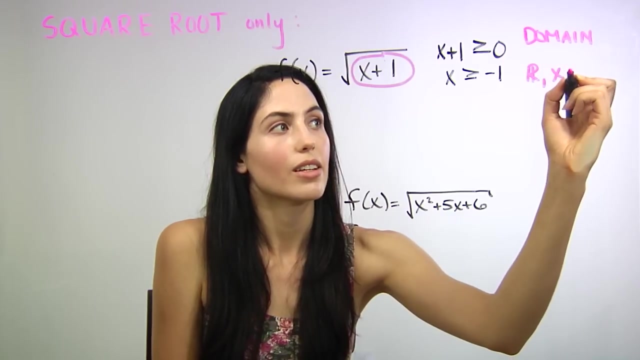 or 0. So what's underneath must be greater than or equal to 0. And you're going to solve that normally, as you would solve any inequality, And you get the restriction: x is greater than or equal to negative 1. So your domain would be all real numbers: x greater than. 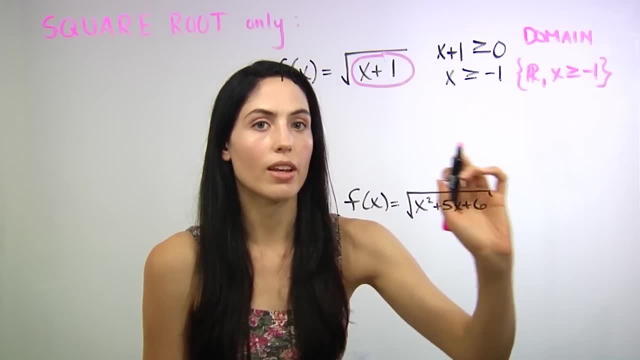 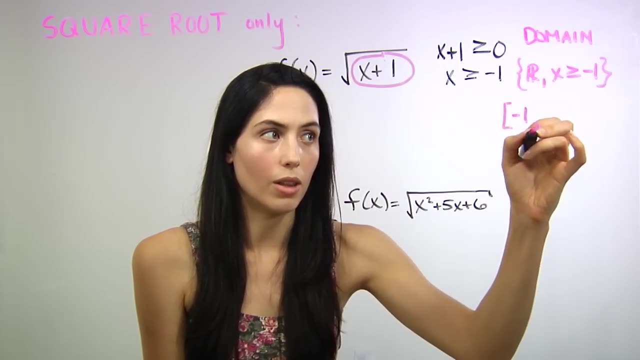 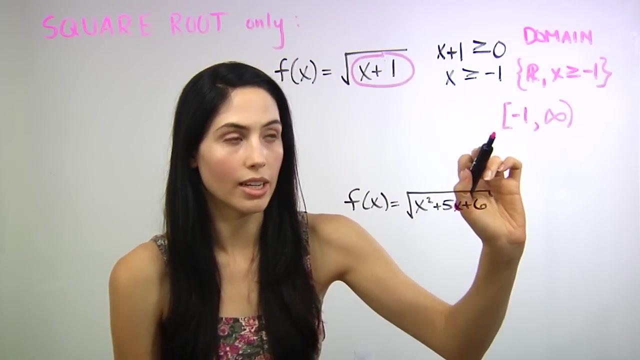 or equal to negative 1.. Or you can write an interval notation as everything from negative 1 all the way up to infinity. Notice that I used a square bracket for negative 1 because we're including negative 1.. And everything all the way up to infinity parentheses. 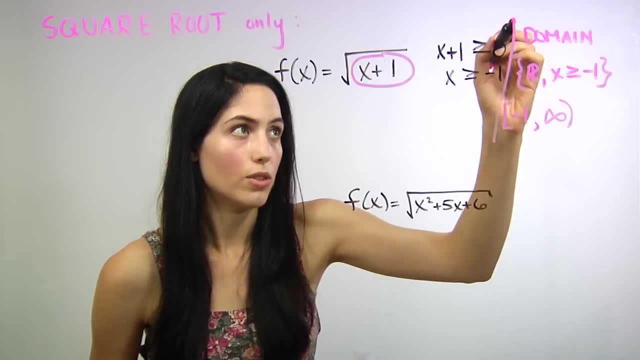 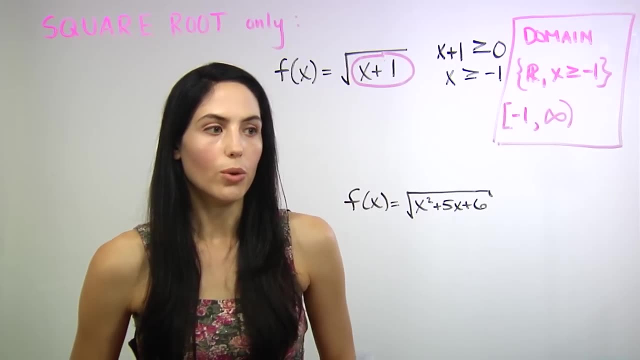 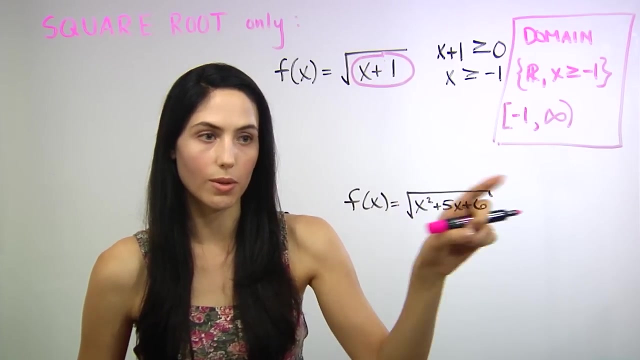 So either of these ways is fine as notation for the domain. OK, let me show you quickly also an example with a quadratic expression under the root. So here we have x squared plus 5x plus 6 underneath a square root symbol. 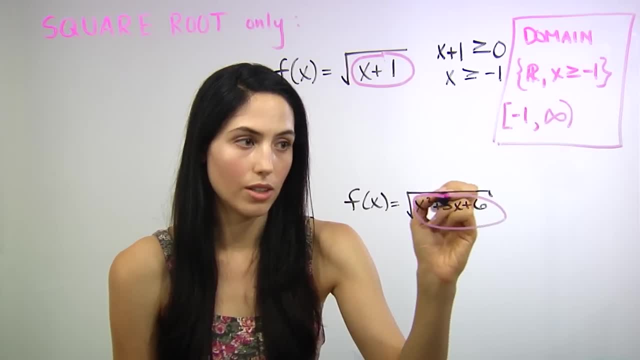 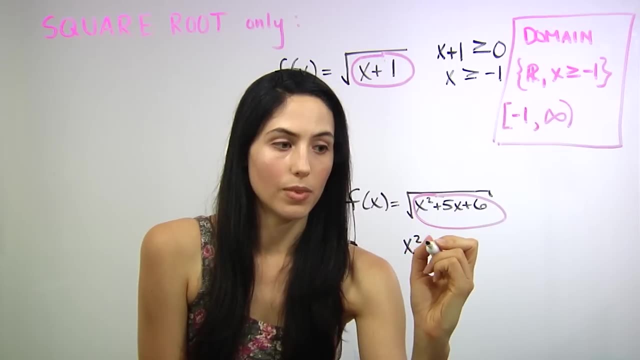 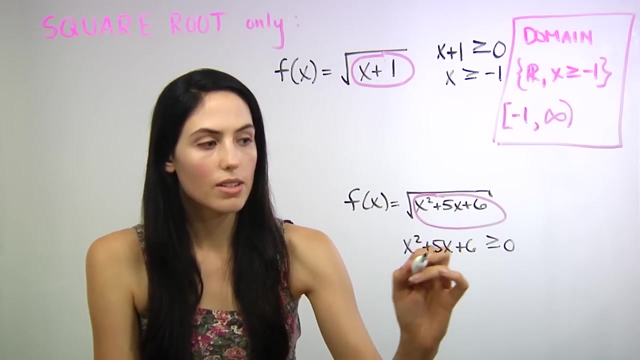 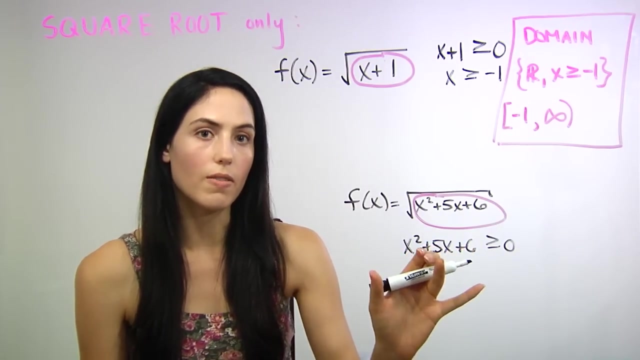 You still do. just take the expression underneath the root symbol and require that it be greater than or equal to 0.. OK, you need to solve this inequality. It's a quadratic inequality which is more complicated than the last example. If you don't know how to solve that, you 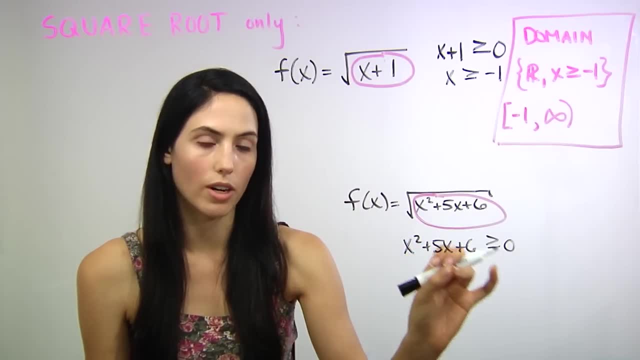 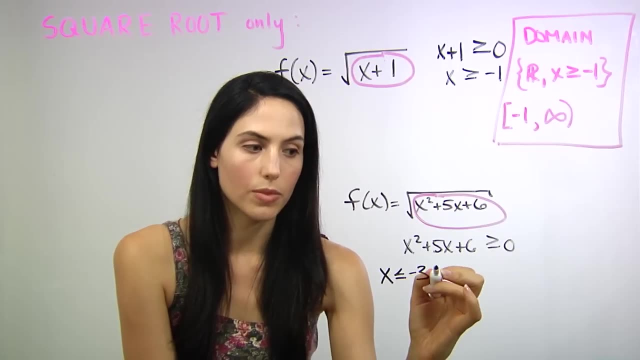 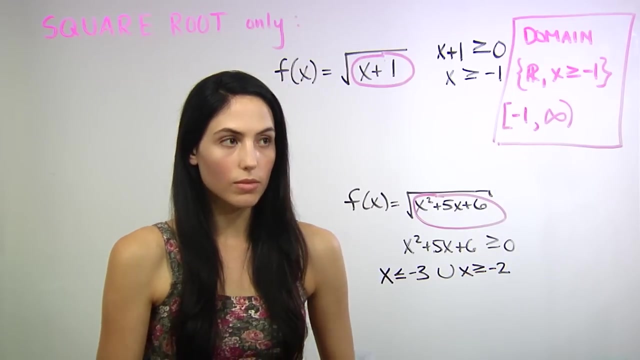 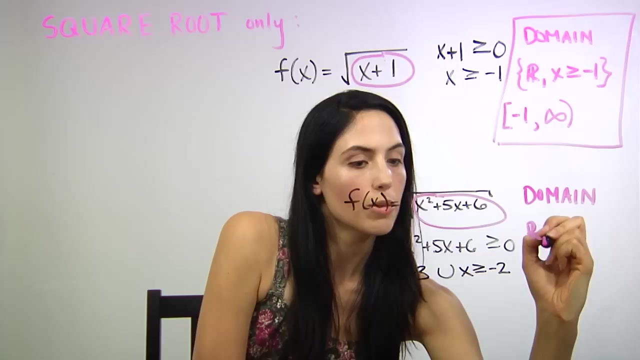 can look it up somewhere else. But once you have solved this quadratic inequality, you will get that x can be less than or equal to negative 3, or x can be greater than or equal to negative 2.. So your domain you can write either as all real numbers. 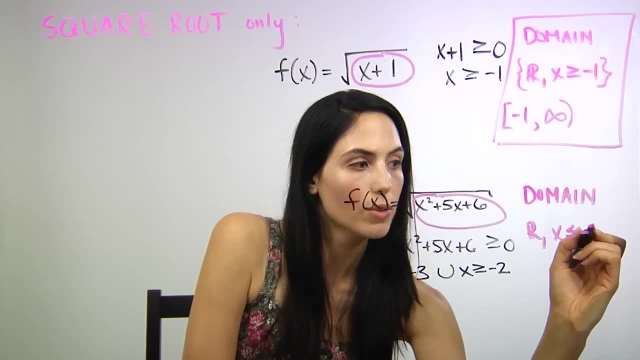 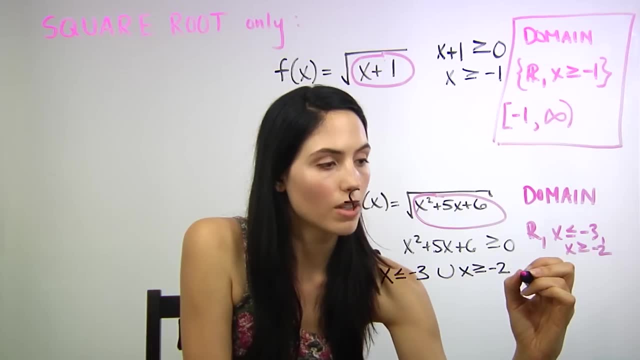 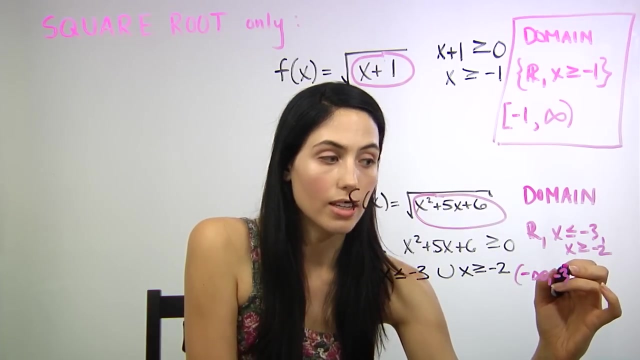 but x less than or equal to negative 3.. Or x greater than or equal to negative 2.. If you were going to write this in interval notation, it would look like everything from negative infinity all the way up to negative 3, including negative 3.. 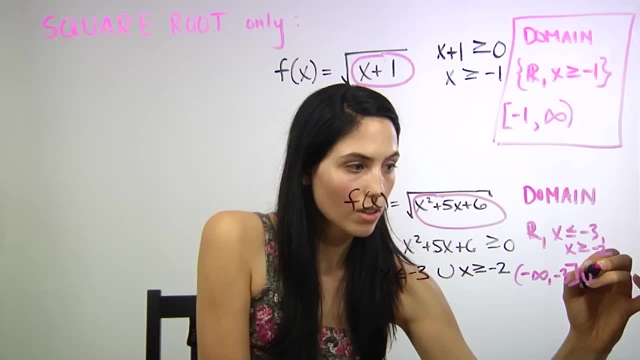 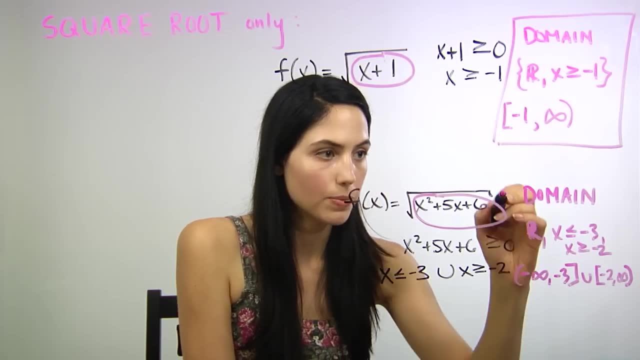 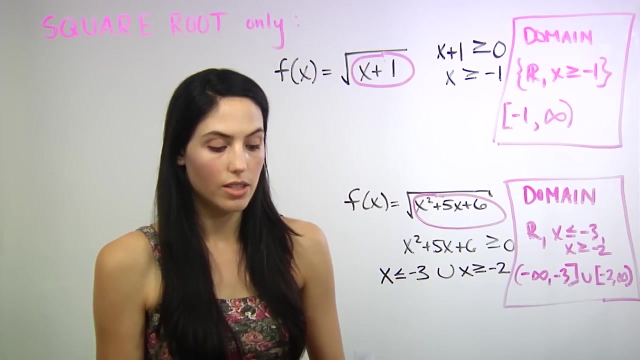 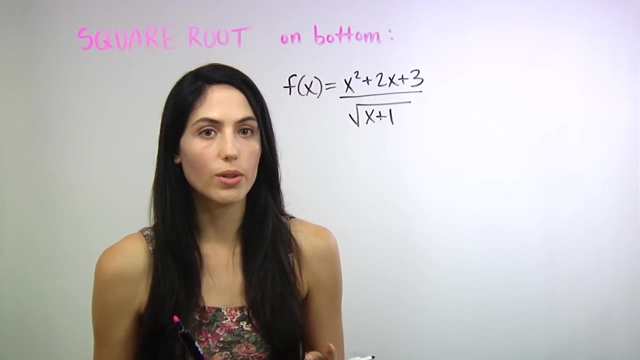 And everything from negative 2 all the way to positive infinity. So e to the power of negative 3.. x greater than or equal to negative 2.. So either of those ways are fine to write your domain answer. OK, if you have a square root in the bottom of your fraction. 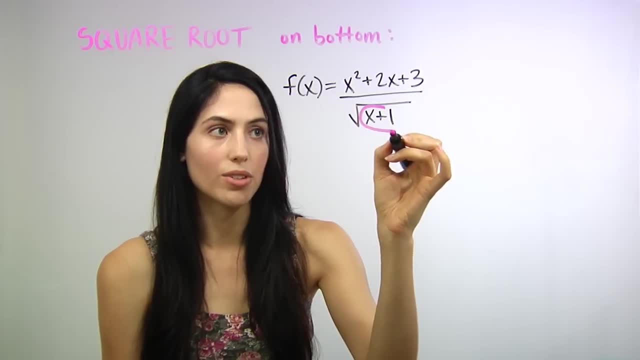 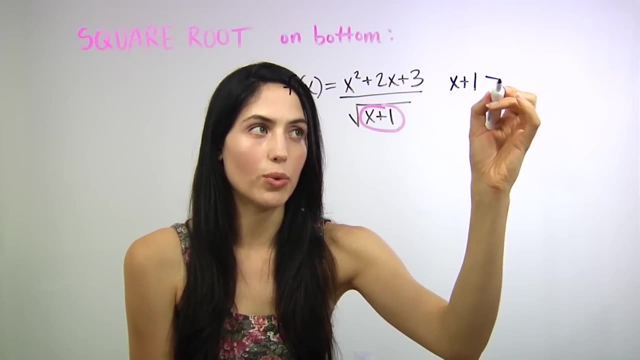 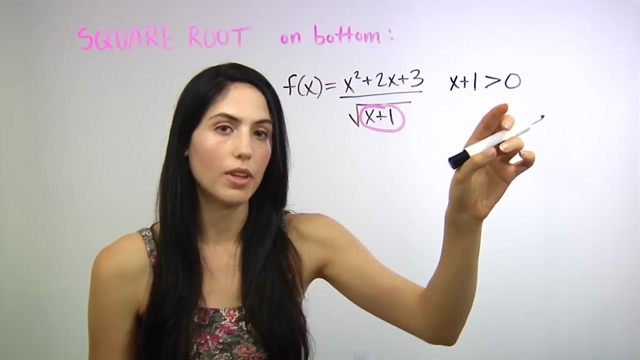 all you need to do is take the expression under the root x plus 1, and set it greater than 0.. Now, usually with a square root, we would set it greater than or equal to 0. But we can't have the denominator equal 0.. 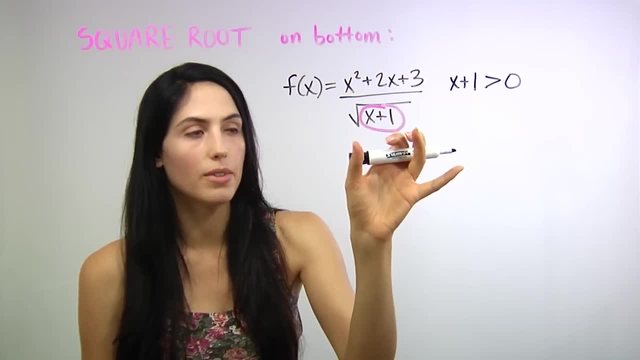 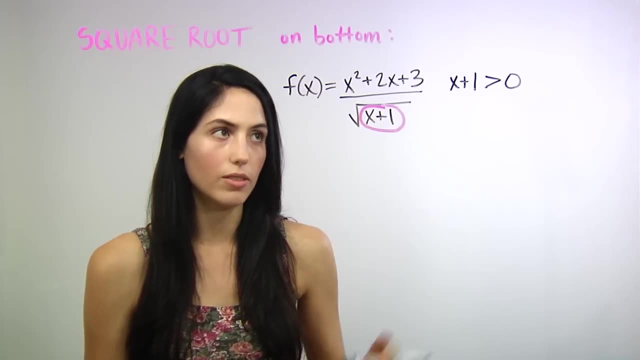 So we leave that part out. So if you see the square root in the bottom, all you need to do is take the expression under the root and set it greater than 0 and solve. So in this case you subtract 1 from each side. 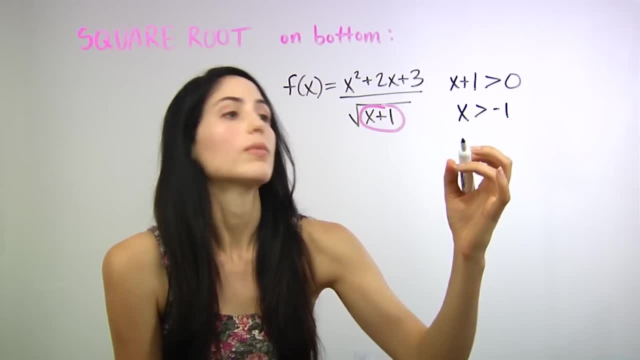 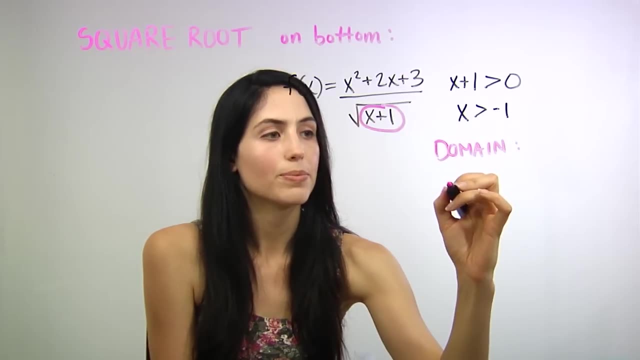 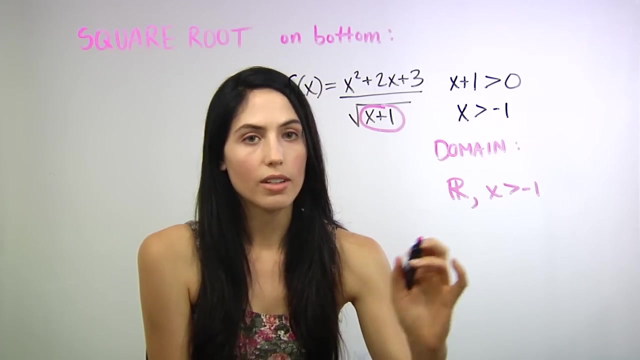 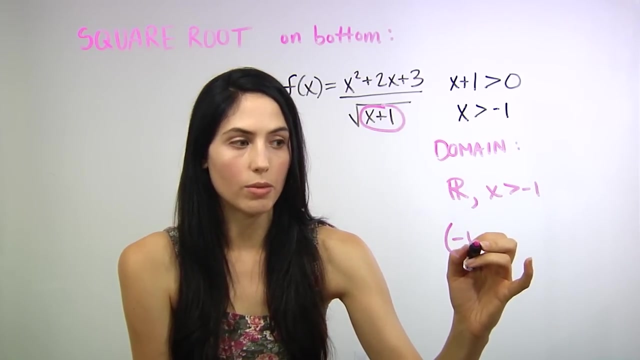 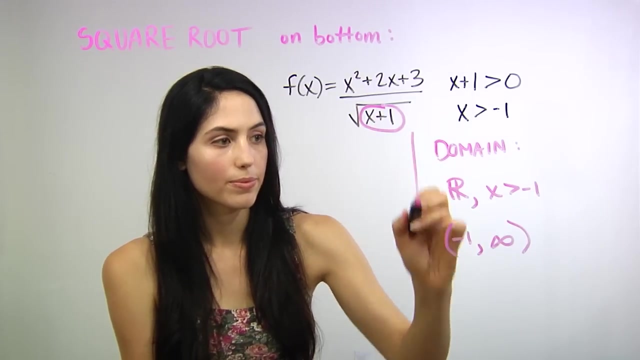 And you would get that x is greater than negative 1.. So your domain It would be all real numbers: x greater than negative 1.. Or if you wanted to use interval notation, you would write parentheses: negative 1.. Everything from negative 1, not including negative 1, all the way up to infinity. 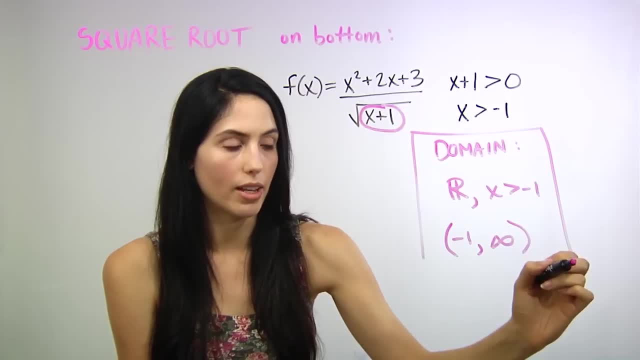 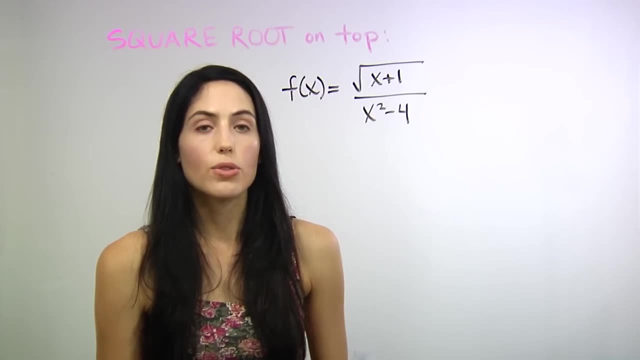 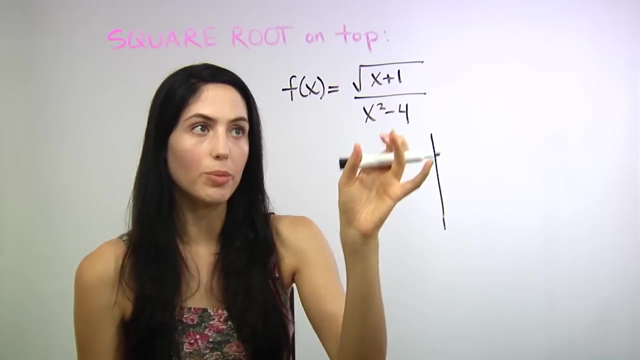 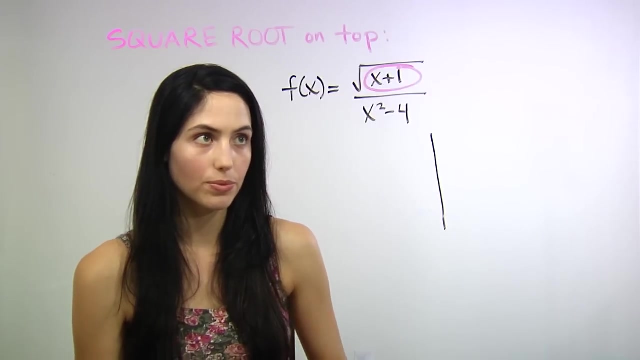 So either of these ways is fine to write your domain answer. Thank you, OK, if your square root is in the top of your fraction, you'll have two restrictions. The first one will be that what's under the square root has to be greater than or equal to 0.. 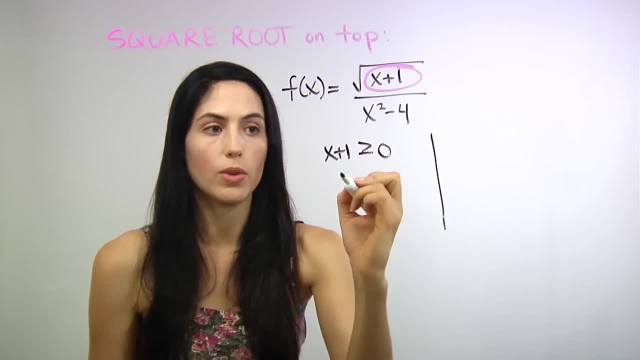 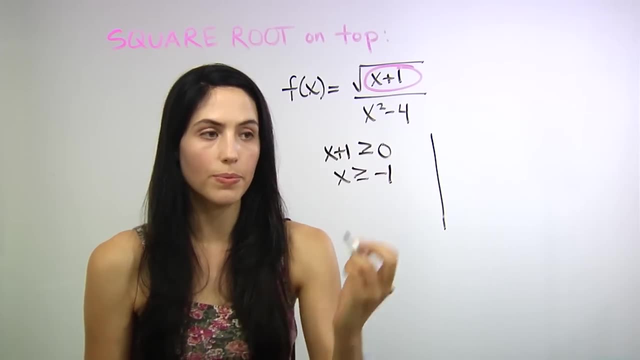 So x plus 1 greater than or equal to 0. And when you solve that by subtracting 1 from each side, minus 1, minus 1, you get x greater than or equal to 0. So that's greater than or equal to negative 1..